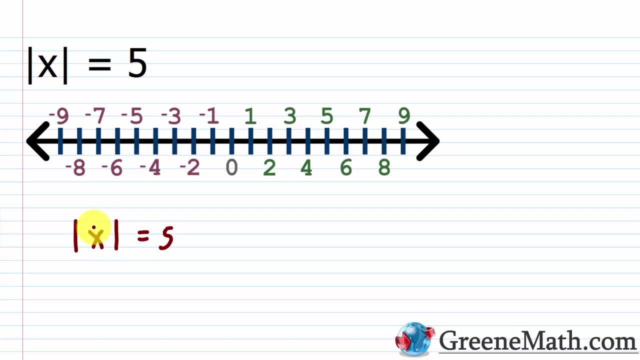 meaning. I want to find the distance between that number and zero on the number line, and it should be equal to five. Well, what numbers have an absolute value of five? Well, it's only going to be five and negative five, right? So five and negative five. okay, So that's. 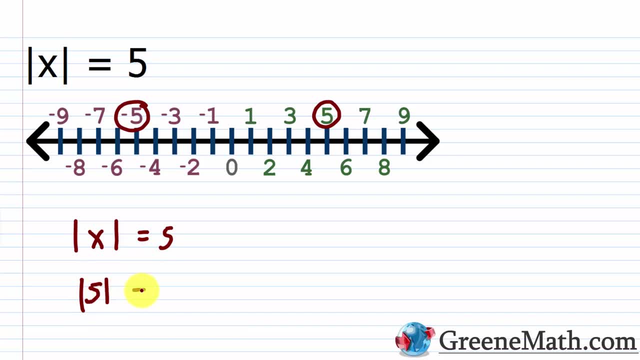 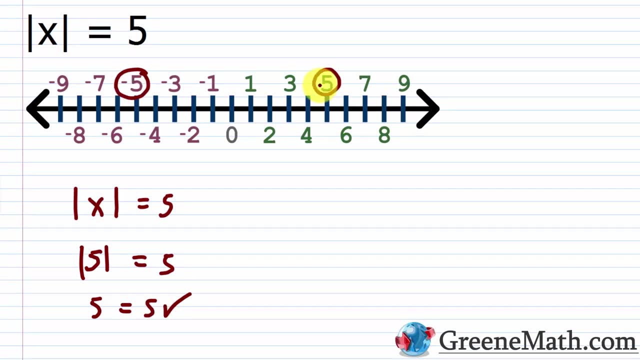 what I can plug in for x. If I plug in a five there and I evaluate, I get five equals five. That's true, But again, that's not the only solution, because negative five, the opposite of five, also has an absolute value of five. So if I plugged in a negative five for x, you would get 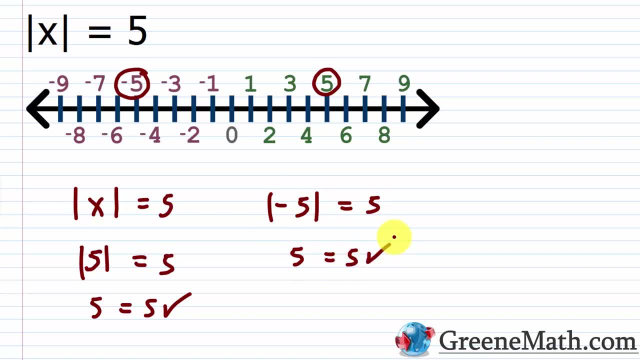 five equals five as well, which is also a true statement. So what ends up happening? is we're going to say that our solution for this equation is going to be what It's going to be- that x could be equal to five, And then we have that keyword or that we talked about in the last lesson, with: 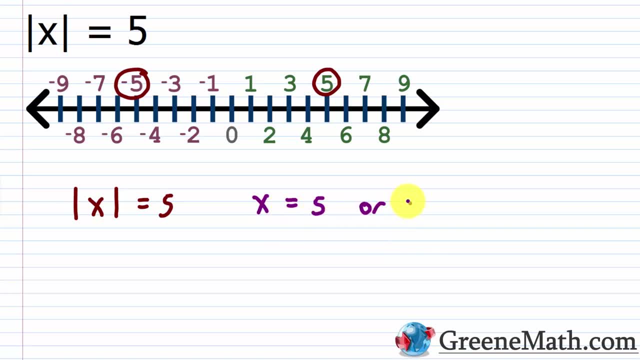 compound inequalities. So x equals five or x equals negative five. Again, the or just tells me that either works. If I plug in a five here- take the absolute value- I get five. five equals five. that's true. If I plug in a negative five, I get five. five equals five, that's true. If I plug 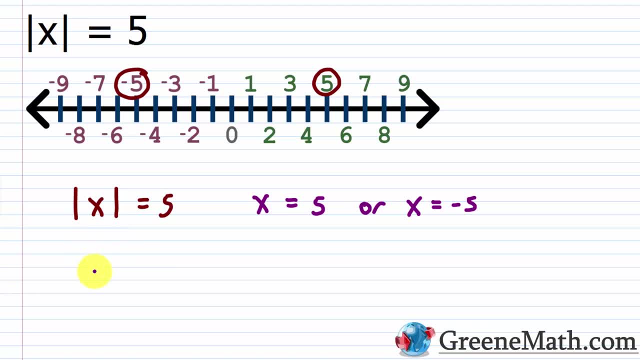 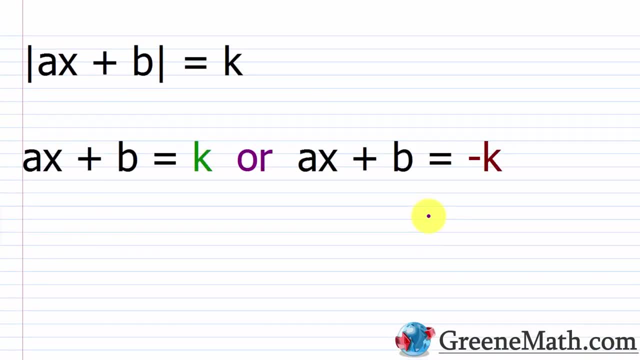 in a negative five. absolute value of negative five is also five. five equals five. that's also true. So either one works. That's why we use the or keyword. Now, in most cases, we're not going to get something as simple as the absolute value of x equals some number. We're going to have some 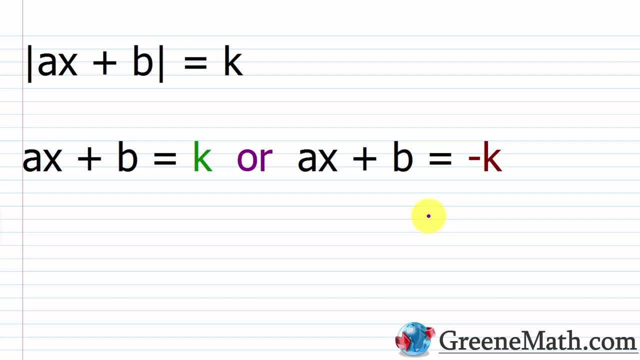 absolute value of an expression equal to some number, or later on we'll see things get more complicated than that. But essentially, if you have an equation in this format, you have the absolute value operation isolated on one side, with an algebraic expression inside. 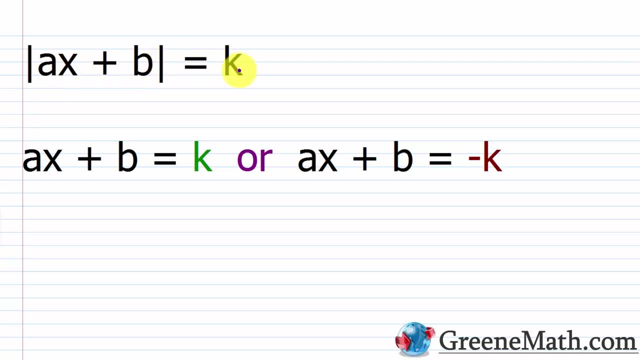 the absolute value bars and it's equal to some non-negative number like k. then we can go ahead and set up a compound equation with or. We can say that this guy right here, the ax plus b, could be equal to k, or ax plus b could be equal to the negative of k. Now it's hard to understand this. 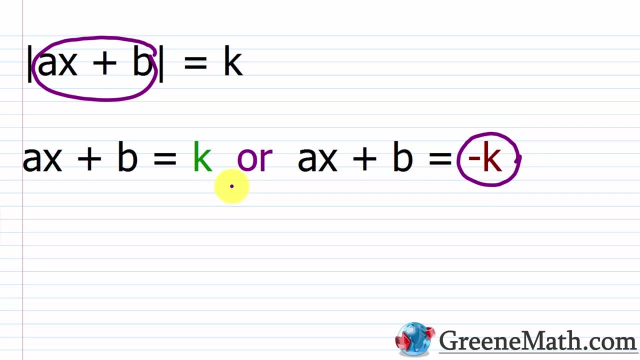 when you look at it in this generic formula. but I want you just to jot this down in your notes anyway, And let's look at the first example. We're going to look at the first example and we're going to kind of relate back to this. So we have the absolute value of x minus three is equal to four. 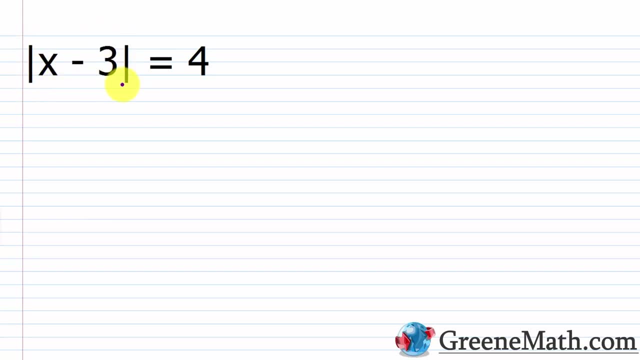 So you see that you have the absolute value operation isolated on one side. you have some non-negative number on the other. Okay, so we're good to go there. So, essentially, what my formula told me to do was to take this expression here, so x minus three, and set it equal to this number. 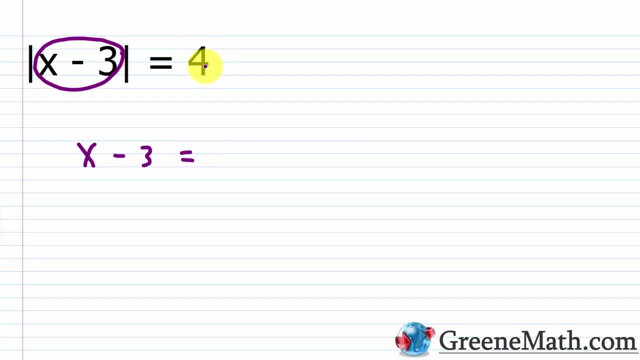 so equal to k. Remember, in this case, k is just four, so equal to four. Then, or you take your expression again, so x minus three could be equal to negative four. Okay, remember you said negative k, now it's just negative four. Now, why does this thought process work? Well, think about it. If I 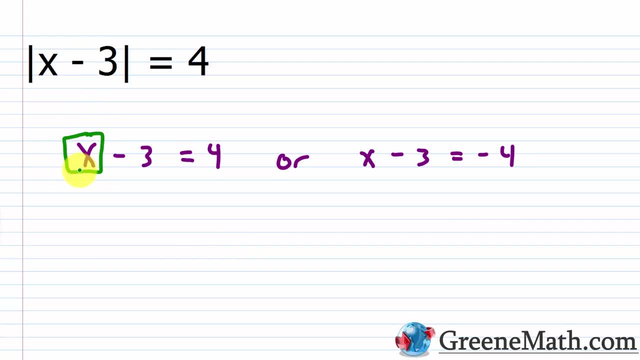 find a value for x that when I plug it in here and I subtract away three, it's going to give me four. Basically, I'm going to be evaluating the absolute value of four and that is four, So I'm good to go there. Alternatively, if I find a value for x, then when I subtract away three, I get 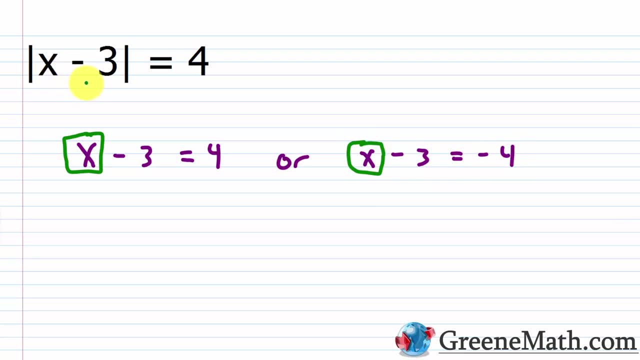 negative four. Well, I'm going to be evaluating the absolute value of negative four, which is also positive four. So that's what I'm looking for. I'm looking to get a result, inside of the absolute value bars here, of either four or negative four. It doesn't matter which one it is, because in each case, 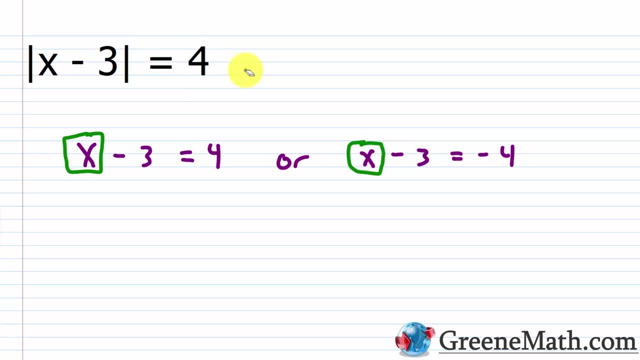 I will get a value of four. So let's go ahead and solve this really quickly. On this one, I would just add three to each side of the equation. I'm going to get that x is equal to seven. For this one, I'm going to add three to each side of the equation and I'm going to get. 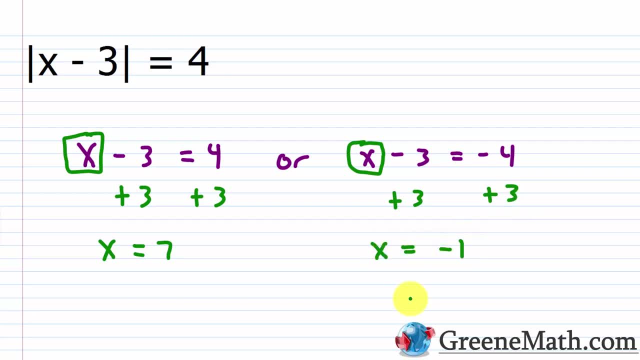 that x is equal to negative one. So let's check these. It's very easy to do, So I'm going to plug in a seven for x here, So I would have the absolute value of seven minus three is equal to four. So seven minus three is four, So I 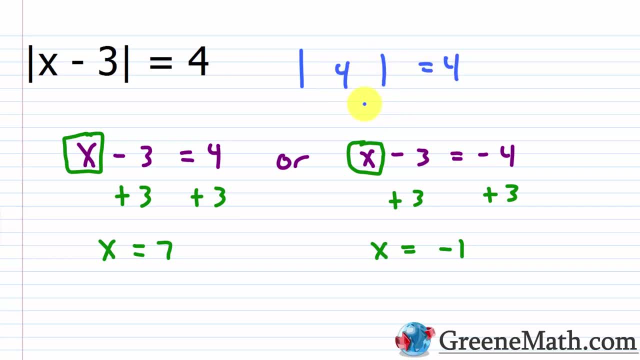 would have the absolute value of four equals four, And of course that's true. Four does equal four. So that's a big check. Okay, so that works. Now let's check the other scenario. We have x equals negative one. So if I plug in a negative one for x right there. so negative one minus three, we're. 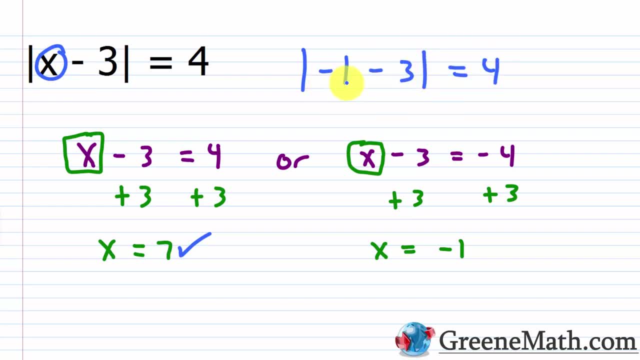 taking the absolute value of that. So I'm going to plug in a negative one for x and I'm going to get that This should be equal to four. Negative one minus three is negative four. So you'd have the absolute value of negative. four is equal to four and we know that's true, right, The absolute value. 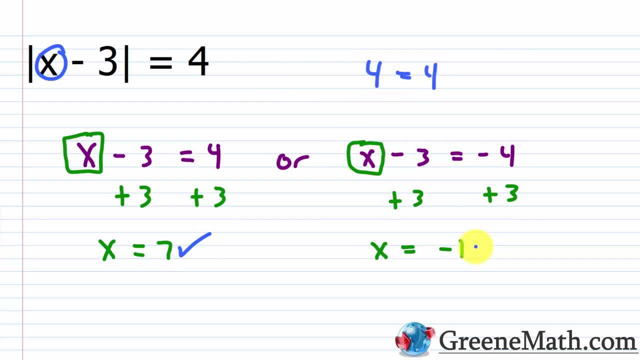 of negative. four is four, So you get again: four equals four. So this one's a big check too. So you can see how that ends up working. right, You take this expression right here, this guy, and you set it equal to this number and then the negative of that number. 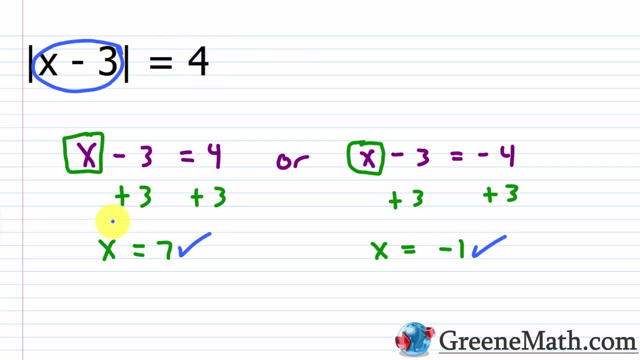 you solve those two equations, you kind of put it together with that keyword or, and then you're going to have your solution. So there's a few different ways to notate the solution. You can kind of remove these check marks. You don't need them anymore. You can just put an. 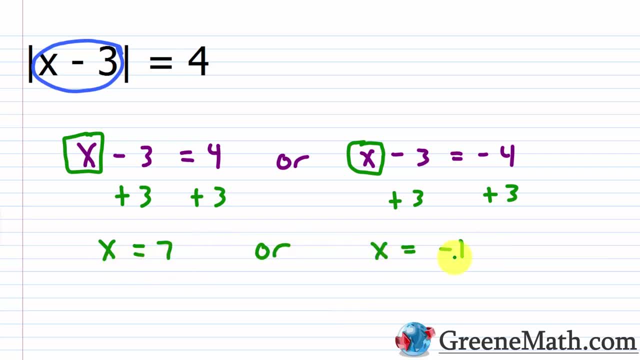 or there between them. So x equals seven or x equals negative one. That's fine. You can use the solution set notation and say: you have negative one and seven as the elements, or basically solutions that work for your equation. And then, lastly, you could also do this: You could say: 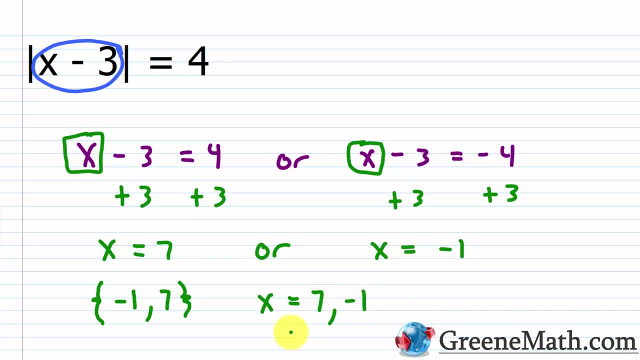 x equals seven comma negative, one right. Lots of different ways. Notate this, but just make sure that you're indicating that each one is a solution to your equation. All right, let's take a look at another one. So we have the absolute value of five x minus. 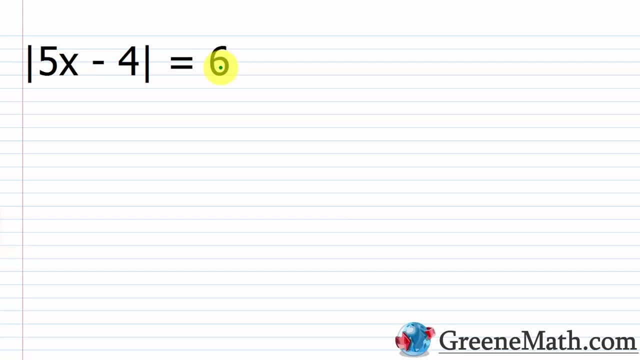 four is equal to six. So again, we're following the same thought process. We're going to take this expression inside the absolute value bars. So five x minus four, we're going to set it equal to six, and we're going to have, or we're going to have: five x minus four is equal to the negative. 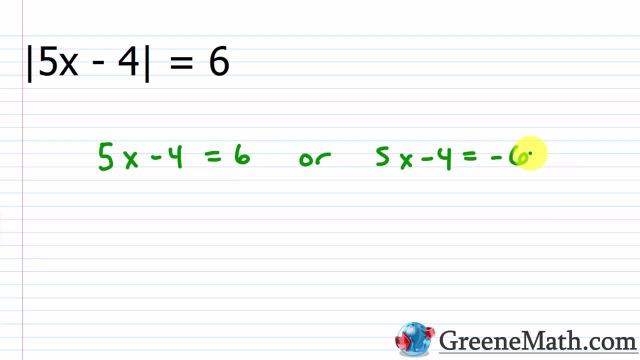 of six. okay, So what we're going to do is we're going to set it equal to six and we're going to add four to each side of the equation here. That's going to cancel. I'll have five. x is equal to ten. 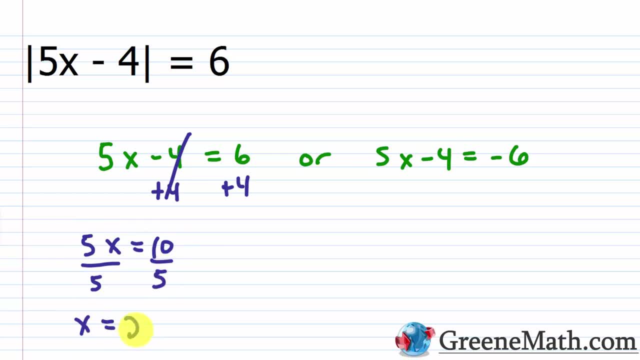 Divide both sides by five and I'll get that x is equal to two. Over here, I just want to add four to each side. That's going to cancel. I'll have five. x is equal to. you'll have negative two. 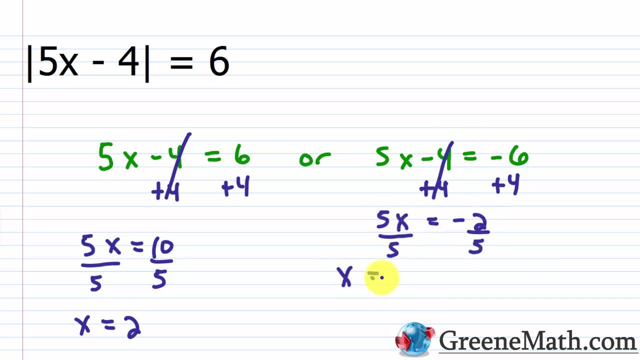 Divide both sides by five and you'll have that x is equal to negative two-fifths. All right, so let's erase these. So I'm going to go ahead and say that x is equal to two or x is equal to negative two-fifths. 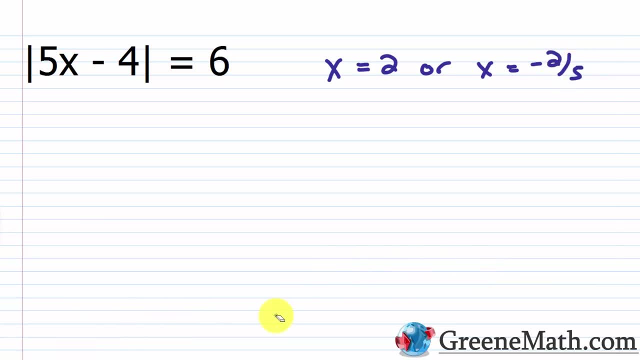 like that. Again, you can write it that way. You can use the solution set notation. A lot of books do that. Or you can also just say that x equals two comma negative two-fifths right. Each is a solution. Now again, if you want to check this, you could plug a two in for x. You can also plug. 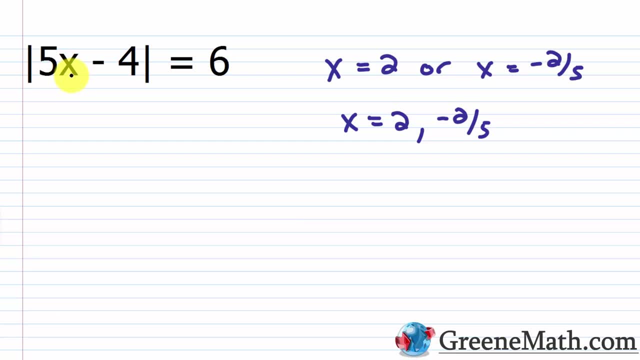 a negative two-fifths in for x and you would see that the left and the right side are equal. So let's go ahead and check it. So the absolute value of five times two and then minus four is equal to six. So five times two is. 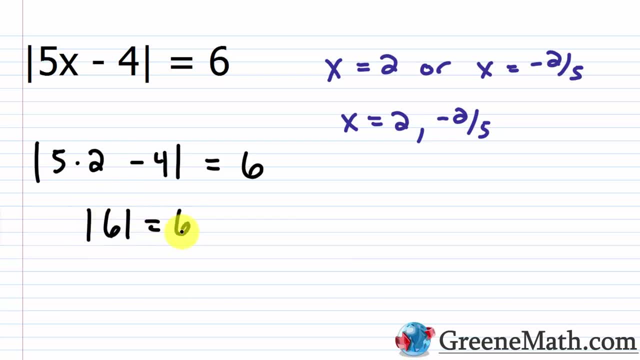 ten. Ten minus four is six. The absolute value of six equals six. So six equals six. So yeah, that's true. You can check that one off. Then the other one is negative two-fifths. So negative two-fifths, So five times negative two-fifths. the fives would cancel You'd have. 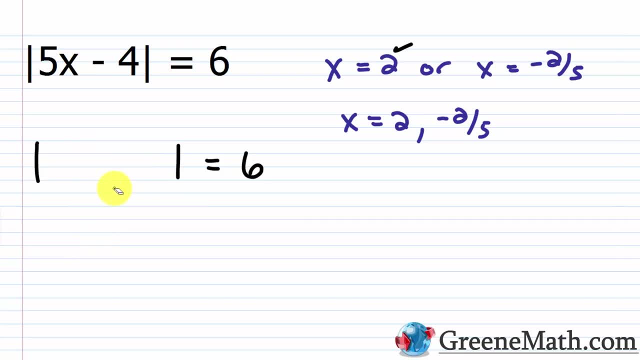 negative two minus four, which is negative six. So you basically have the absolute value of negative six, Which we know is six. So six equals six here. So this one checks out as well. So again, x equals two or x equals negative two-fifths, Let's look at one that's a little bit more complicated, It's just: 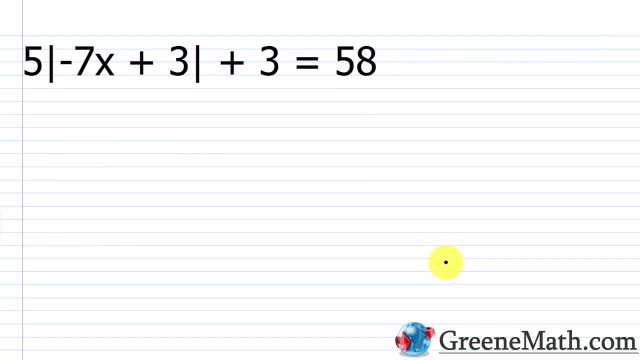 more complicated because you don't have the absolute value operation isolated on one side. So we have five multiplied by the absolute value of negative seven x plus three plus three equals 58. So your goal, if you get something like this, is to isolate the absolute value operation. So 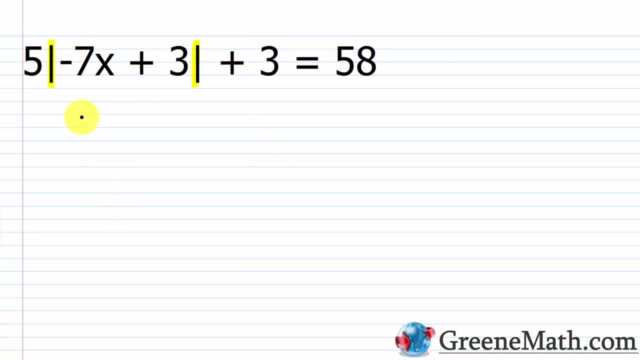 how can we do that? It's very, very easy. You just think about what's being done to that absolute value operation. You have multiplication right, You're multiplying by five and you have addition Three is being added to it. So let's go ahead and subtract three away from each side to start. We'll get rid of. 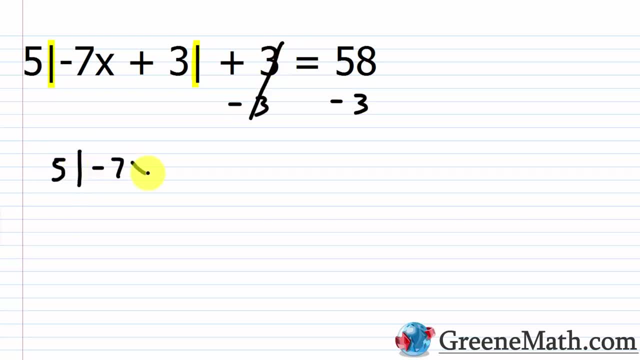 that We'll have five times the absolute value of negative. seven x plus three, And this equals 58 minus three is just 55. Now I can just divide both sides by five. So I divide both sides by five and this would cancel with this. 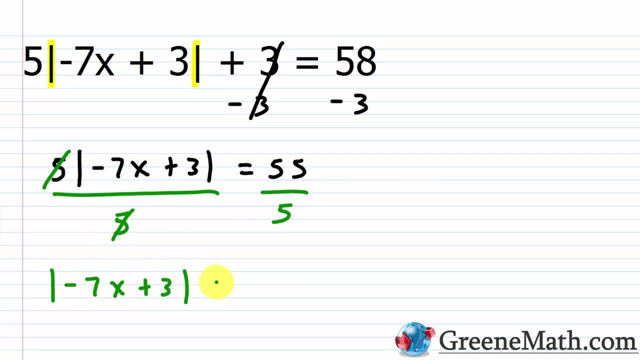 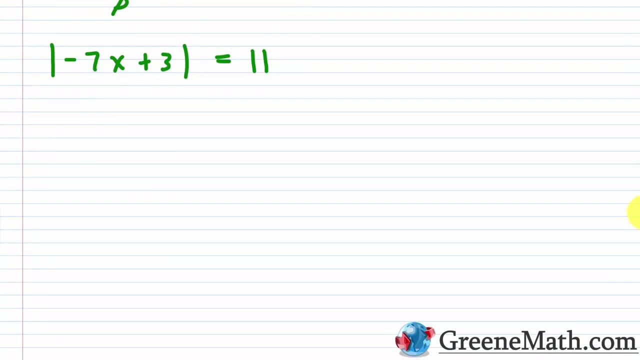 So the absolute value of negative seven x plus three is equal to 55 over five is 11.. So now I have it in the format that I've been looking at And again, once I have it like this, it's very, very easy. I take my expression: So negative seven x plus three, I set it equal to 11.. And then I say: 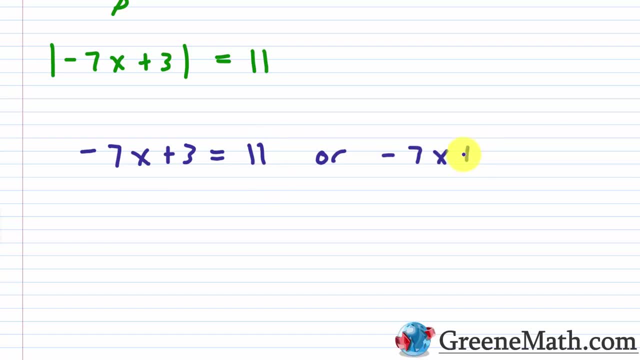 or I take my expression. So negative seven x plus three, I set it equal to negative 11.. Okay, Just solve each one Very, very simple. So I'm going to subtract three away from each side of the equation. I'm going to get negative seven x is equal to 11 minus three is eight. 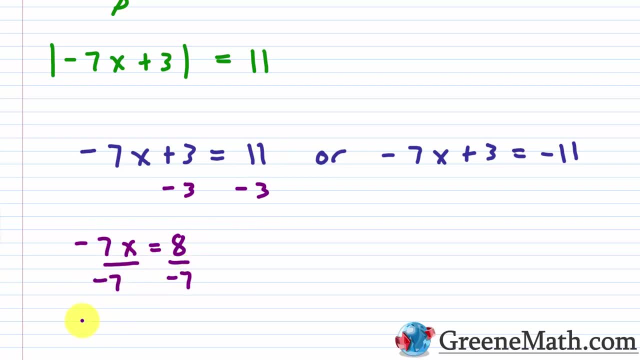 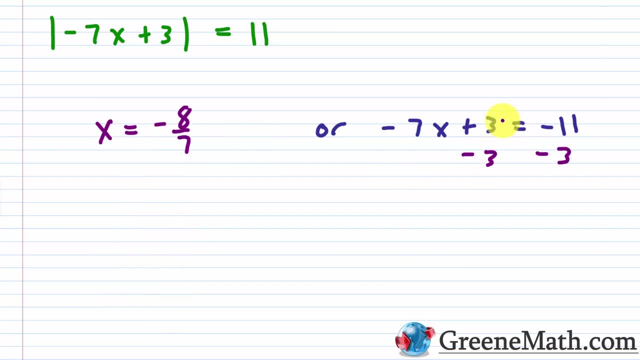 Then I'm going to divide both sides by negative seven And I'm going to get that x is equal to negative eight sevenths Over here. let me subtract three away from each side. That cancels. You'll have negative seven. x is equal to negative 14.. Divide each side by negative seven. 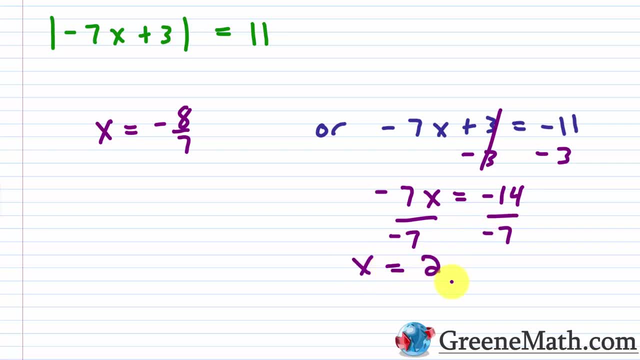 And you get that x is equal to positive two. So let me erase this. So again, x equals two. So you can leave this as your solution. Again, you can write it in solution set notation. You can put the comma. There's a zillion different things. you can do whatever. 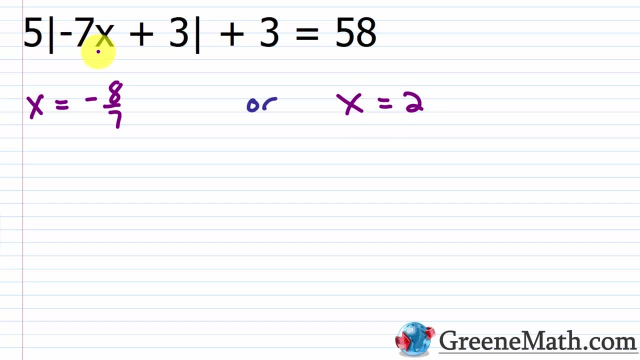 you're more comfortable with. So let's go ahead and check this real quick, And then all the rest of them. I'll leave that up to you to check them on your own. So I would have five multiplied by the absolute value of, I'd have negative seven times negative eight sevenths. So we know that. 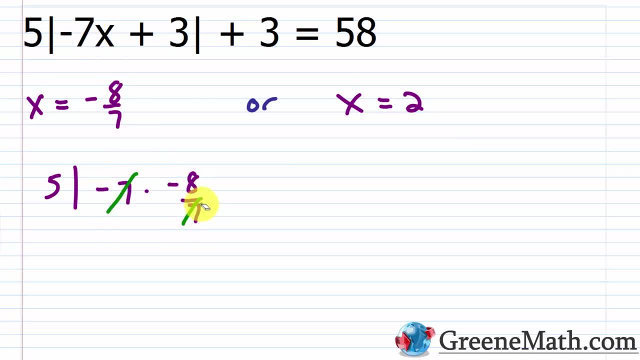 this would cancel. with this, The negatives would cancel. So I'm basically just going to have an eight sevenths. So I'm going to have negative seven times negative eight sevenths, So I'm going to have eight there. So I'd have eight plus three, which is just 11.. So then plus three equals 58.. 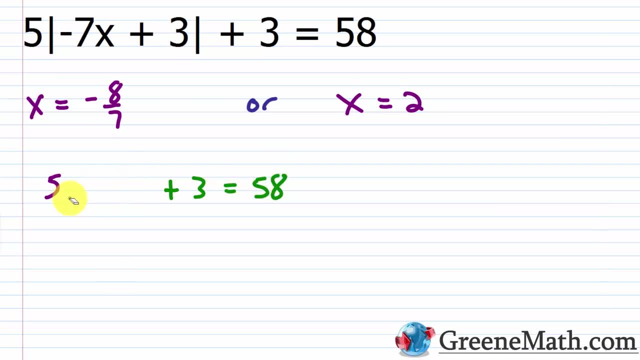 So the absolute value of 11 is 11.. So you have five times 11 there, That's 55. And then 55 plus three is 58. So this one's good to go Over. here you have the two that's going to be plugged in for. 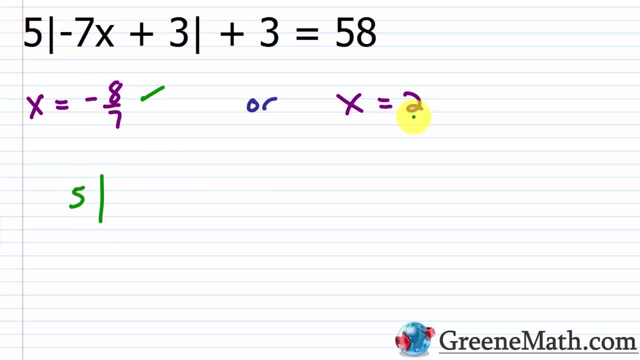 x. So five times the absolute value of negative. seven times two is negative 14.. Negative 14 plus three is negative 11.. But again, because I'm taking the absolute value there, it just becomes positive 11.. So five times 11, then plus three equals 58. We already know that's true Five times. 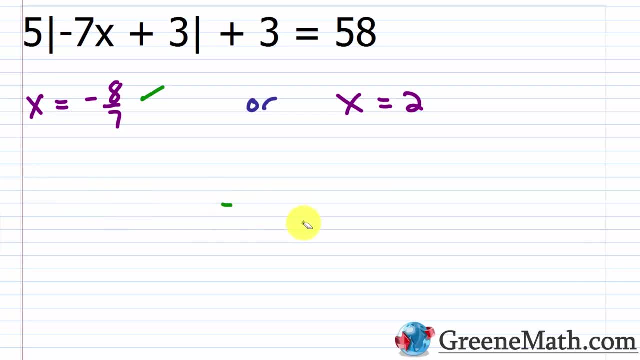 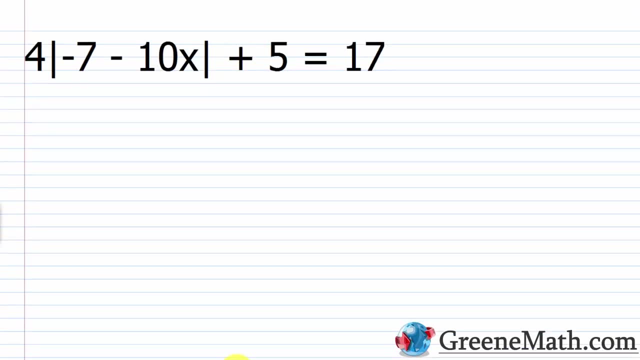 11 is 55.. 55 plus three is 58. So we're good to go. in each case, Again, our solution is: x equals negative eight sevenths, or x equals two. All right, let's take a look at another one. 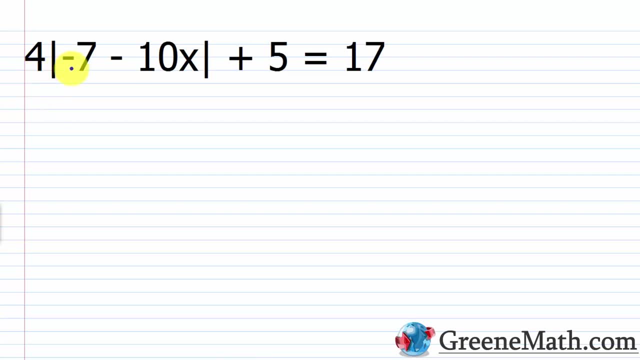 So suppose we had four multiplied by the absolute value of negative seven minus 10x. Then we had plus five and this was equal to 17.. Again, my goal here is to isolate the absolute value operation. So I'm going to take a look at another one. So suppose we had four multiplied by 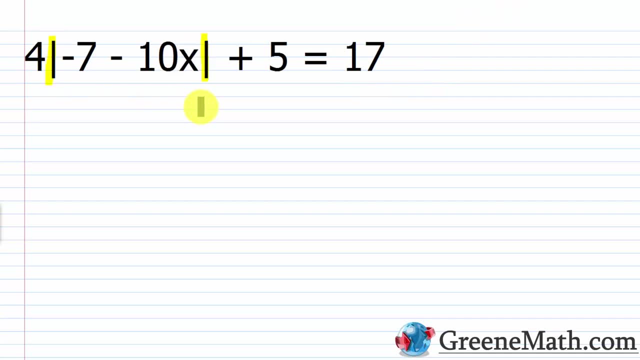 the absolute value operation on one side and then to have a number on the other. Okay, so what I want to do? I want to just subtract five away from each side of the equation to start. So we know this would cancel. So we'll say: we have four times the absolute value of, we have negative seven minus. 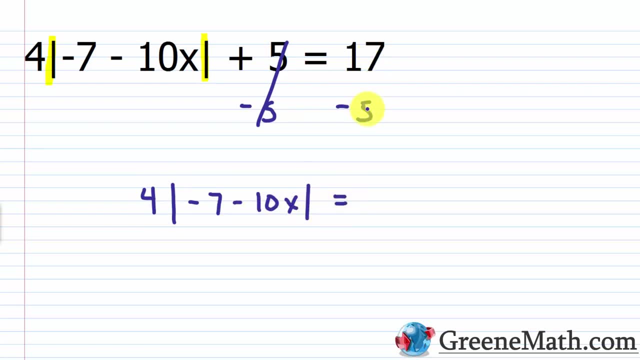 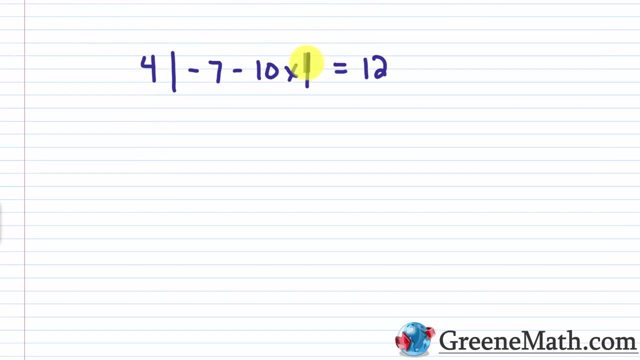 10x, And then this is equal to 17 minus five is going to give me 12.. Scroll down, get some room going. All right, so to isolate the absolute value operation, I have four. that's multiplying it. So all I need to do is divide by the absolute value of negative seven minus 10x, And then I'm going to 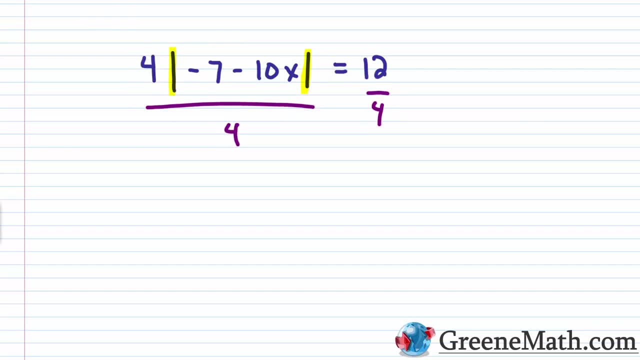 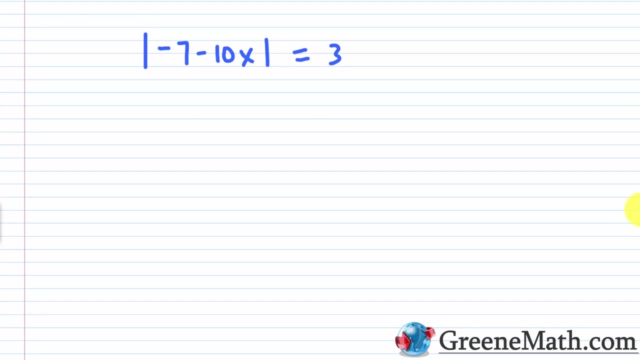 do is divide both sides of the equation by four. So we know that again this would cancel. I'll have the absolute value of negative seven minus 10x. This will be equal to 12. divided by four is three. So now we have this in the format of our absolute value. operation equals some number, So the 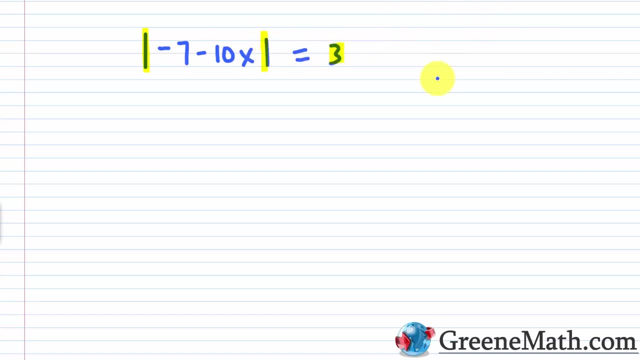 absolute value operation here is equal to some number, So I can set up my compound equation with: or, So I just take the expression inside. In this case it's negative seven minus 10x. I'm going to set it equal to three, Then, or I'm going to take my. 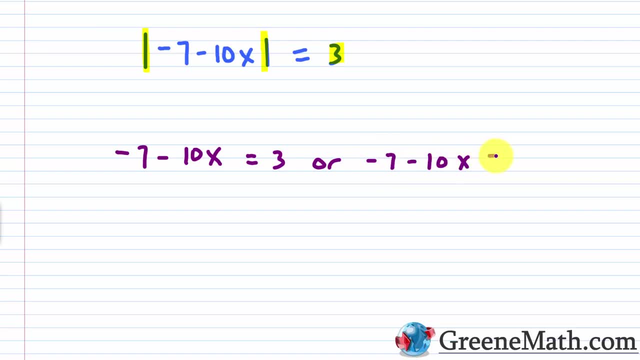 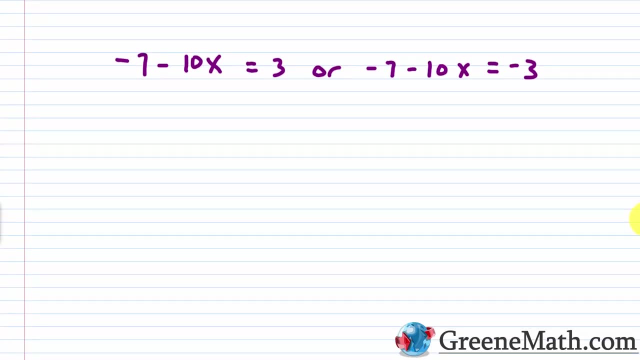 expression inside. So negative seven minus 10x. And I'm going to set it equal to the negative of three, So negative three. And then I'm just going to solve these two equations here And I'll have my solution. So on the left, I'm just going to add seven to each side of the equation, I'll have 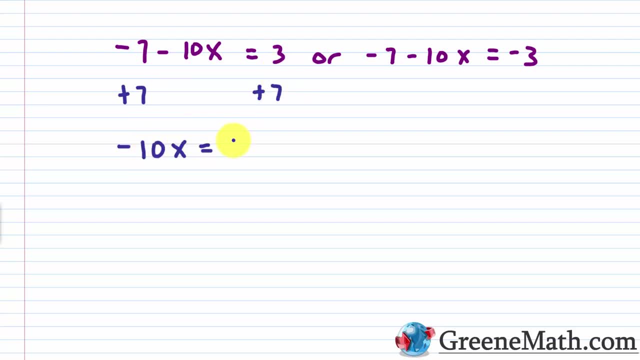 that negative 10x is equal to three plus seven is just 10.. And now we can divide by the absolute value equation by negative 10.. And of course this guy is going to cancel. I'll have: x is equal to 10 over. 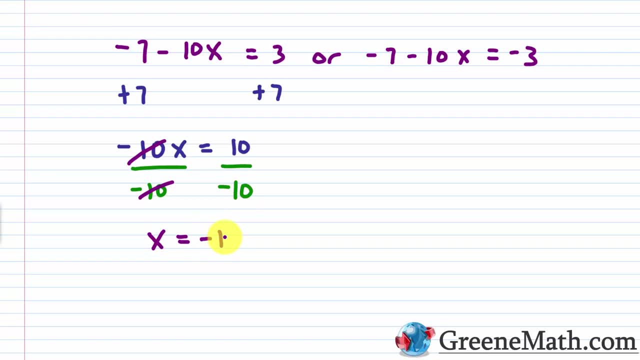 negative 10 is just negative one. So that's one solution. Let's get our other solution over here on the right. So again, I'm going to add seven to each side of the equation. this is going to cancel. I'll have negative. 10x is equal to negative. three plus seven is going to be four. So now let me. 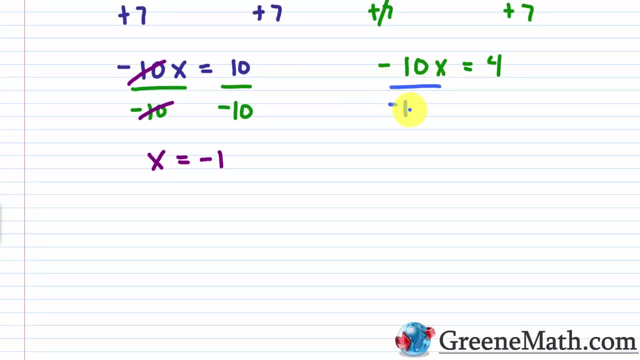 scroll down and get a little bit more room here. If I divide both sides of the equation by negative 10, then this guy right here is going to cancel with this guy and I'll have x is equal to four over negative 10.. We know that's negative. they're each divisible by two. four divided by two is two. 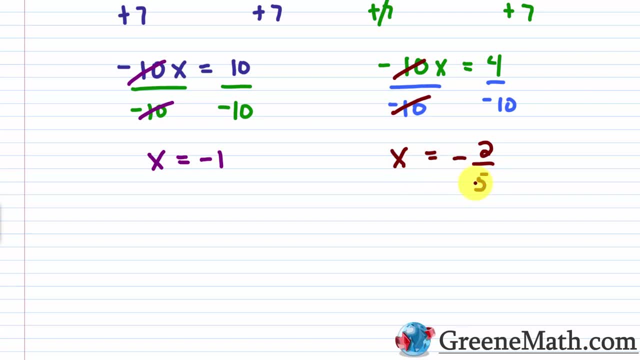 and 10 divided by two is of course five. So I get x equals negative two fifths. So I can write this as x equals negative one, or my keyword, or x equals negative two fifths. Again, you can do the solution set notation, or you can just list them with a comma. whatever you want to do All. 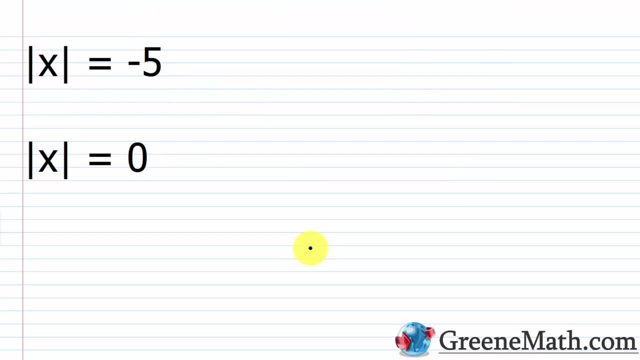 right. so let's take a look at some special case scenarios That come up when we're solving absolute value equations. So the first one we're going to talk about is the situation where you have no solution. So something like the absolute value of x is equal. 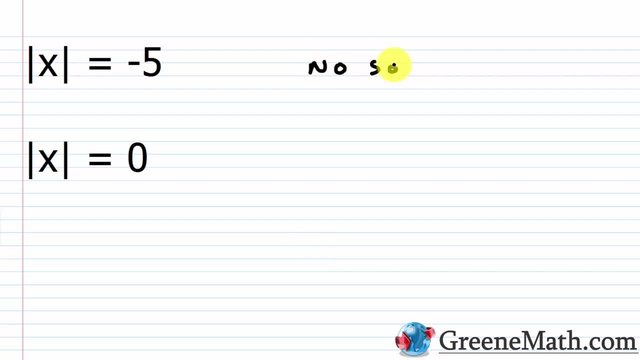 to negative five, this guy would not have a solution. So no solution. Why is that the case? Well, we should know that the absolute value of some real number, x, is greater than or equal to zero. Because if I plug in a zero here, I'd get zero. If I plugged in a negative here, I'd get a. 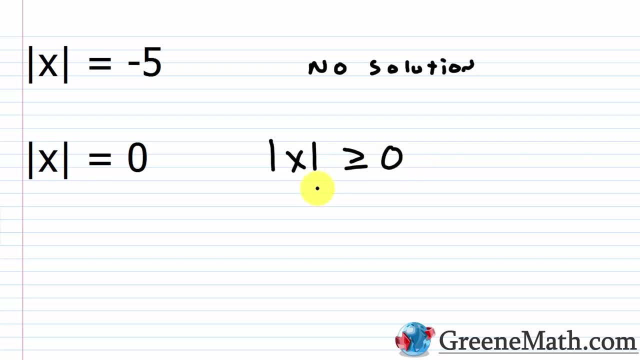 positive, And if I plugged in a positive I would get a negative. So I'd get a positive, And if I plugged in a positive I'd get a positive. Right, This stems from the definition of absolute value. When you take the absolute value of the number, you want the distance from zero to the number. on. 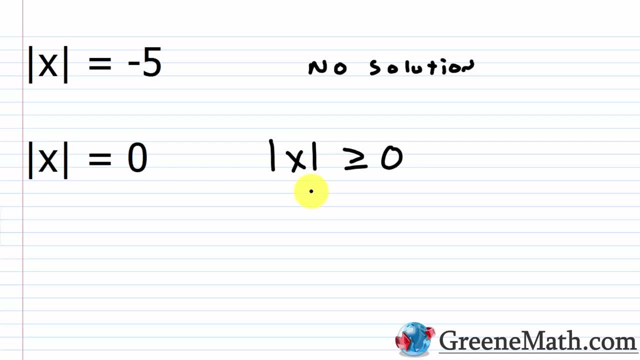 the number line. So if it's zero, it's just going to be zero. If it's some negative, again, you'd get a positive. If it was a positive, it would just be a positive. Okay, so you're never going to get a. 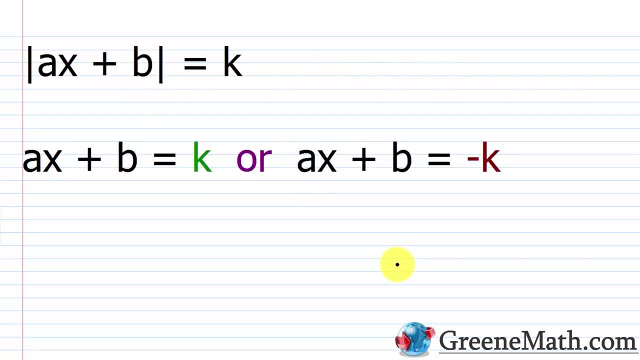 negative result. So this guy would always be no solution. When we go back to our generic formula here, I said earlier that the absolute value of some expression, ax plus B, if this is equal to k, k has to be non-negative. So if you've isolated this guy right here, the absolute value operation. 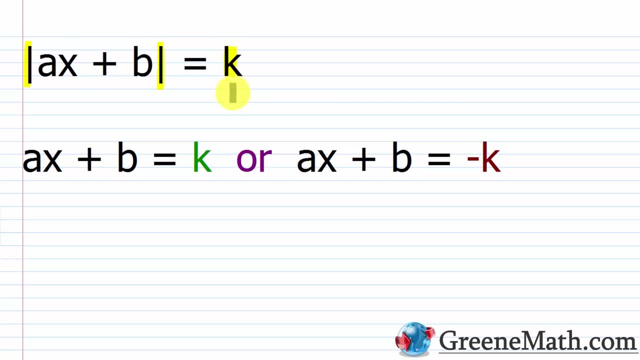 on one side and on the other side you have a negative value, you can stop and say there's no solution. What you don't want to do is say there's no solution before you've isolated the absolute value operation on one side. That can lead to problems, Okay, so you need to make sure. 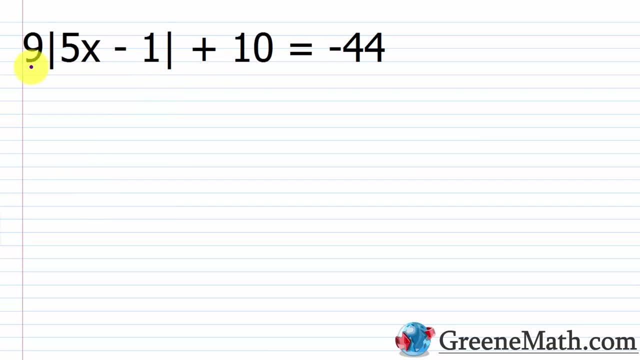 you isolate first. All right, let's take a look at an example. So we have nine times the absolute value of five x minus one. then plus 10 is equal to negative five x minus one. So if I plug in a negative here, I can see that the absolute value of five x minus one is equal to negative 44. So the 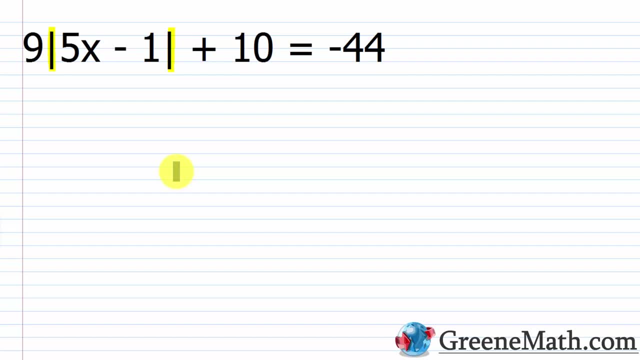 idea here is that we want to isolate the absolute value operation on one side of the equation And then we want a number on the other. But if that number on the other side happens to be negative, we're not going to have a solution. So don't just look at the negative over here on the right hand. 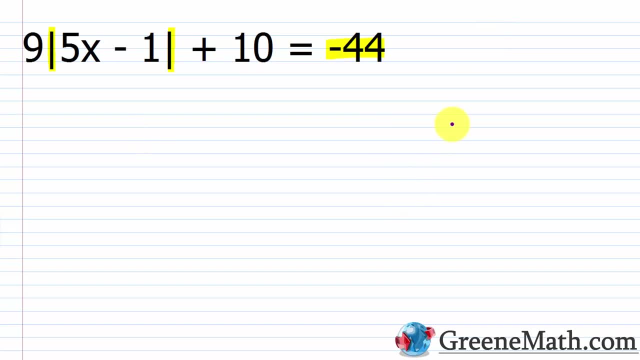 side and assume that this guy is going to be a no solution. to start, You've got to isolate the absolute value operation before you can make that determination. So I'm going to start by just going to cancel this. We'll have nine times the absolute value of five x minus one, And this is 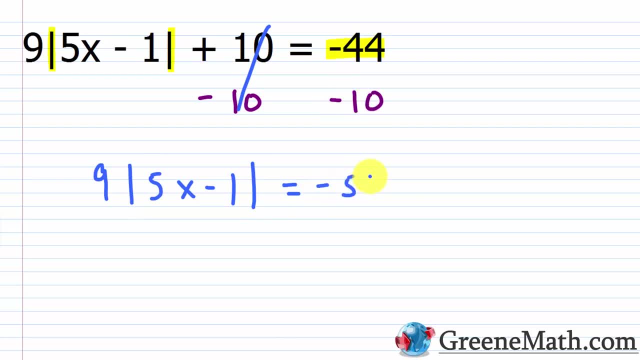 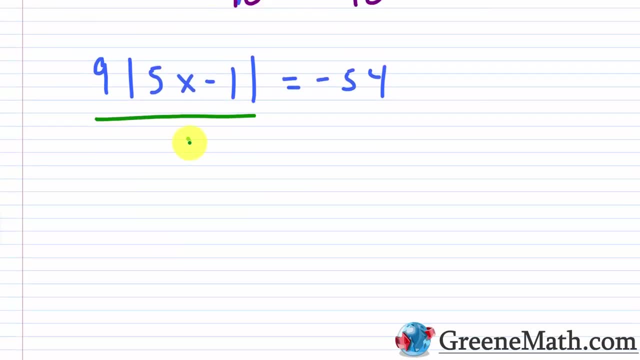 going to be equal to negative. 44 minus 10 is negative 54. So at this point you pretty much know it's going to be no solution, But let's continue. Let's go ahead and divide both sides by nine And of course this will cancel. we'll have the absolute value of five x minus one. 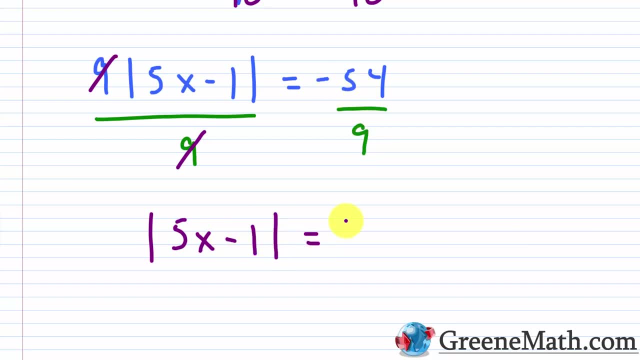 is equal to negative. 54 over positive nine is negative six. So we know at this point there's no solution, So we're going to cancel this And then we're going to have nine times the absolute value of five x minus one is negative 54 over positive nine is negative 64.. So we know. 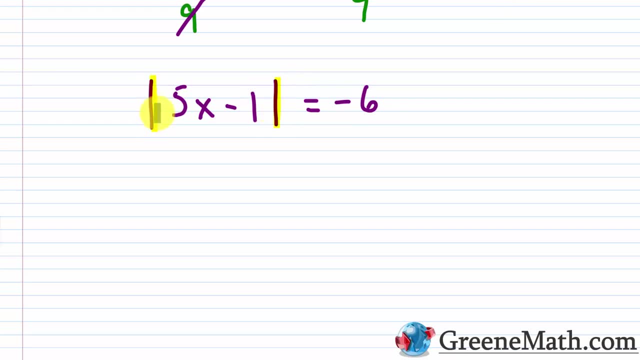 there's no solution. right, There's no solution. We have isolated the absolute value operation on one side and we have a negative number on the other, So we can just say that there's no solution like this. This is what I always do. I just write no solution. A lot of textbooks. 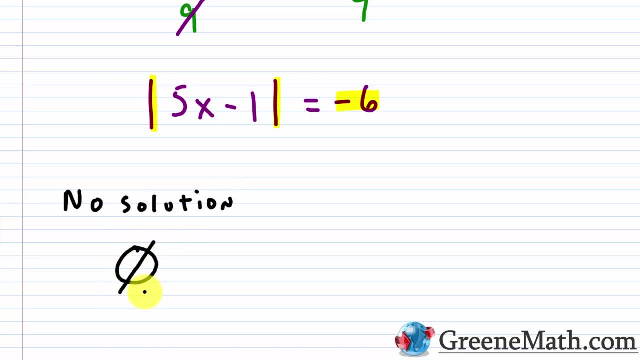 again will use the symbol for the null or empty set, which looks like this: That's fine too, if you want to write that. it's basically anything you want to do. So again, I just want to emphasize here why there's no solution, There's no value I can plug in for x there. 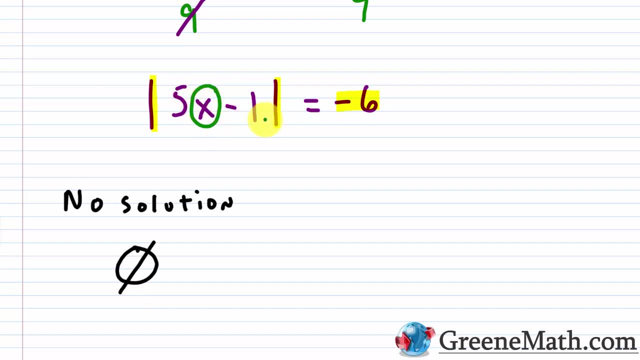 Multiply by five and then subtract away one, and then take the absolute value of it and get negative six. It doesn't matter what this value is. Once I take the absolute value, it's either going to be zero or positive, So it can never, ever ever be negative six. So that's why there's 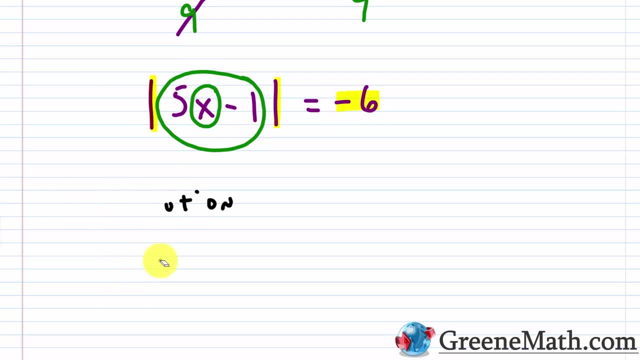 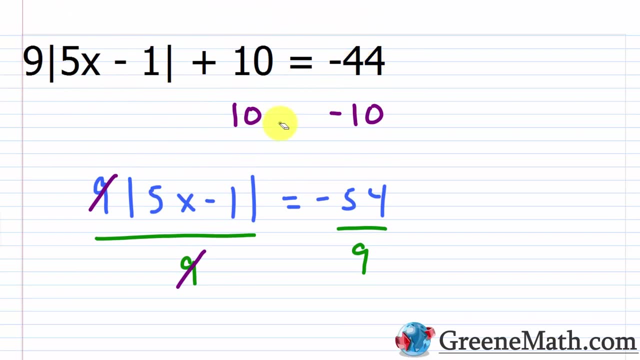 no solution Now. let me show you one thing real quick. I just want to make sure we're crystal clear on this before we move on. If, for example, I change this problem- and I'm not going to go all the way through, but if I change this problem- I'm going to get negative six. So I'm going to get 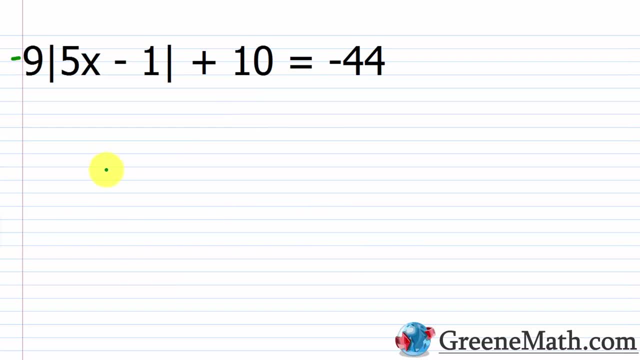 negative seven. If I change this problem to a negative out in front, you will have a solution. Okay, let's work through that real fast. I'm not going to go all the way through, but I'll just show you. If I subtract 10 away from each side here- that would cancel- I'll have negative nine. 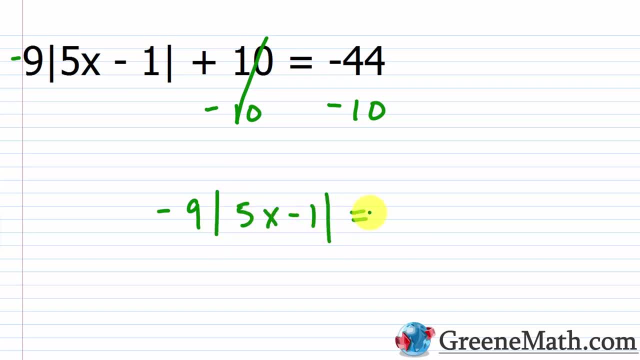 times, the absolute value of five x minus one is equal to negative. 44 minus 10 is negative 54.. Now if I divide both sides by negative nine, what's going to happen? Let's scroll down, get some room. Well, we see that this guy right here cancels with this guy. 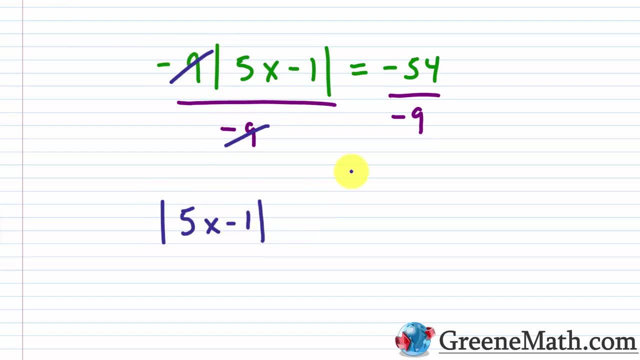 so I've isolated the absolute value of five x minus one. but now negative 54 over negative nine is positive six. So I would have a solution here. I would have to set five x minus one equal to six, and then five x minus one equal to negative six. so I would have that compound equation with or: 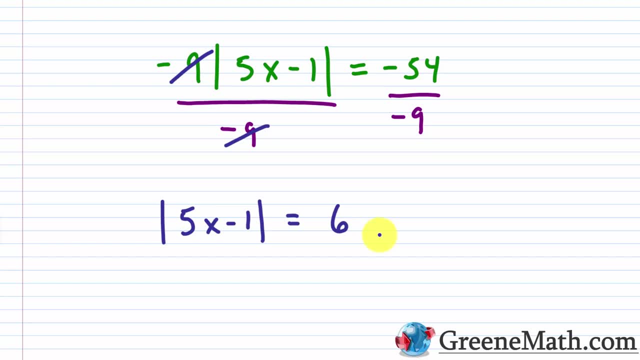 and I would get two solutions there. I'm not going to go through that process, but I'm just making sure that you understand that just because I start with a negative on the right-hand side doesn't mean that I have no solution. You've got to get to the point where you've 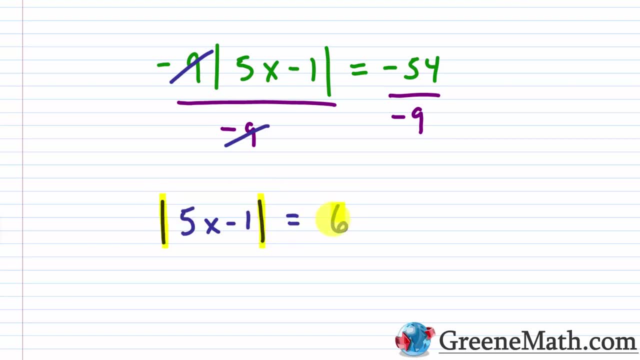 the absolute value operation on one side and a number on the other. If the number is zero, then you're just going to have one solution, which we'll talk about in a minute. If it's positive, you're going to have two solutions, and if it's negative, you're going to have no solution. 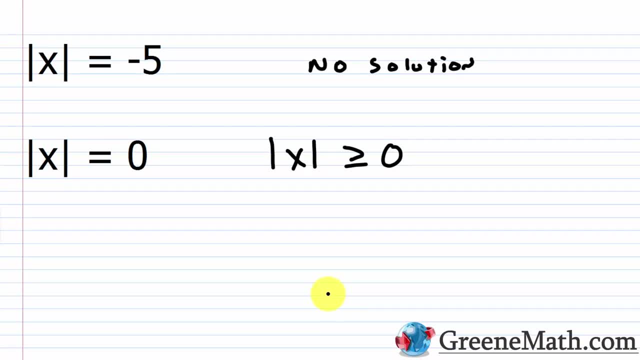 All right, let's think about another scenario we're going to come across. So suppose the absolute value of x was equal to just zero. Well, in this case you're not going to have to set up a compound equation with, or, You're just going to have one equation, The. 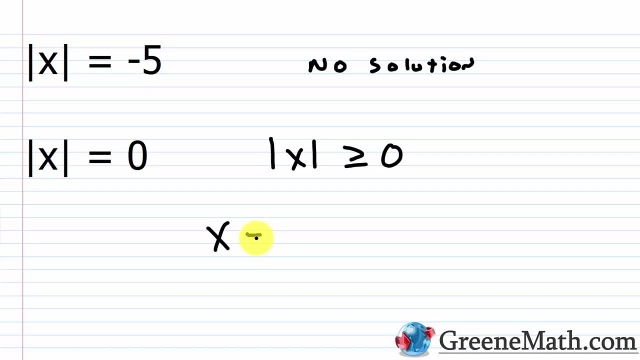 absolute value of x equals zero, You're not going to have to set up a compound equation with or Only if x is equal to zero. Okay, that's the only possible solution there, because the only number that has an absolute value of zero is just zero. Zero doesn't have an opposite. 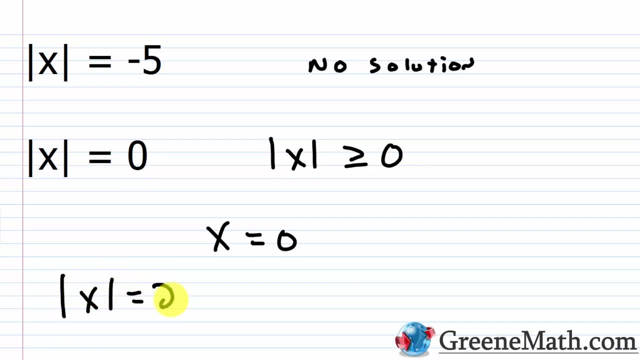 If this was, the absolute value of x is equal to two. again, x could be two or it could be negative two, because each have an absolute value of two. But when you get zero there, you only have one unique number that has an absolute value of zero, and that's just zero. So let's look at this. 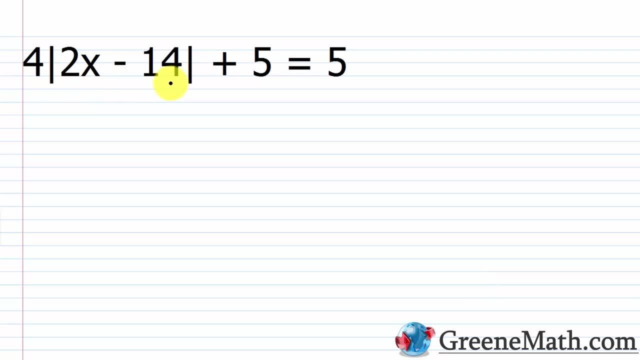 equation here. So we have four times the absolute value of two x minus 14, then plus five is equal to five. So again, our goal is always to isolate the absolute value operation. And when I subtract five away from each side, you're going to immediately see you. 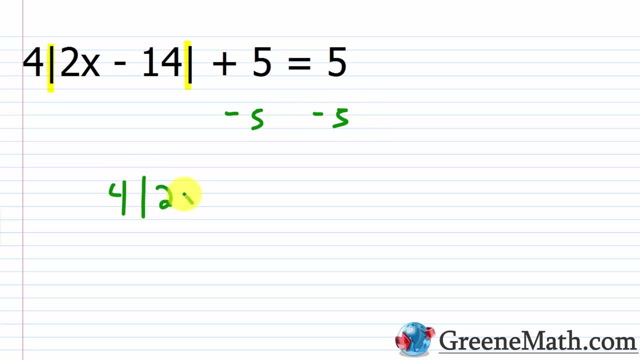 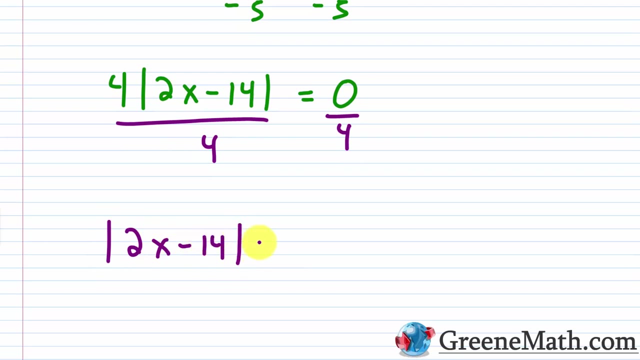 have a problem. You get four times the absolute value of two x minus 14, and this is equal to zero. So if I divide both sides by four, we know zero divided by four is just zero. So I'm going to end up with: the absolute value of two x minus 14 is equal to zero. So this is. 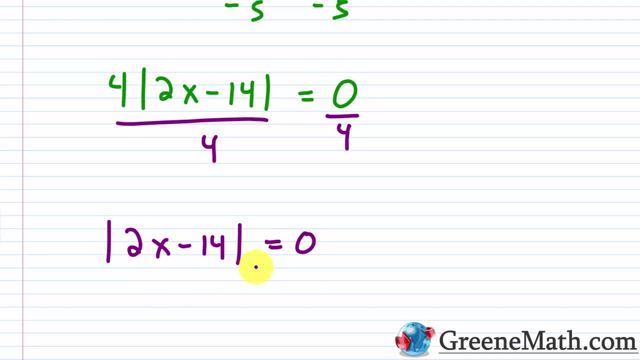 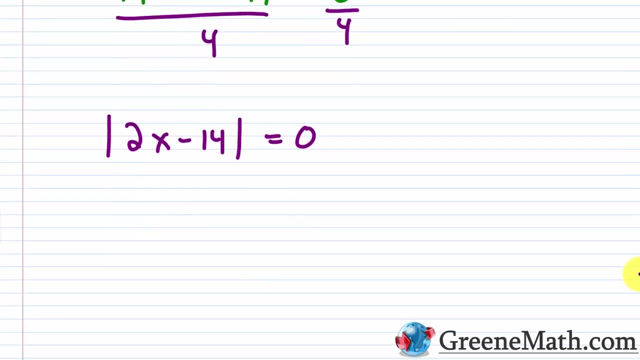 a scenario: okay, You do have a solution here, but you only have one. okay, You're not going to get two. So you need to pay close attention to what to do here. So all we need to do is say that two x minus 14 is just equal to zero. We're just going to solve that equation. So I'm going to add: 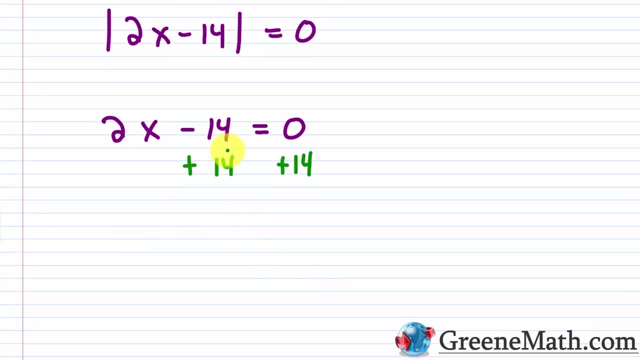 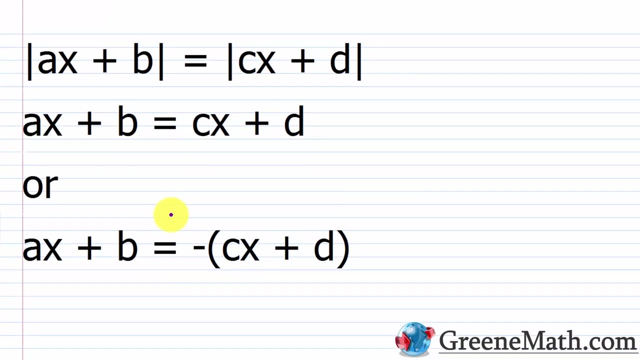 14 to each side, And of course this is going to cancel. We'll have two: x is equal to 14.. Then we're going to divide both sides by two and I'm going to get that x is just equal to seven. So just one solution here: x equals seven. So lastly, let's think about what happens when we 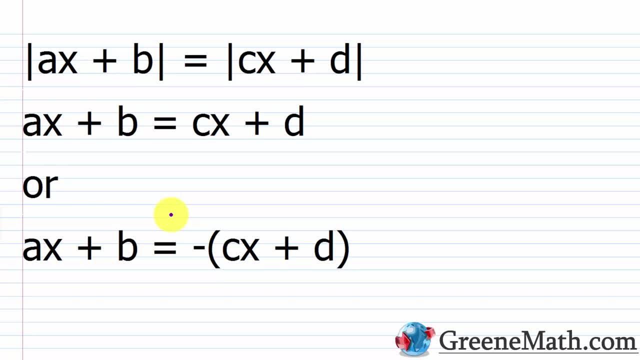 have two absolute value operations set equal to each other. So something like the absolute value of ax plus b is equal to the absolute value of cx plus d. So the way we think about this is two numbers or expressions can only have the same absolute value if they're equal to each other. 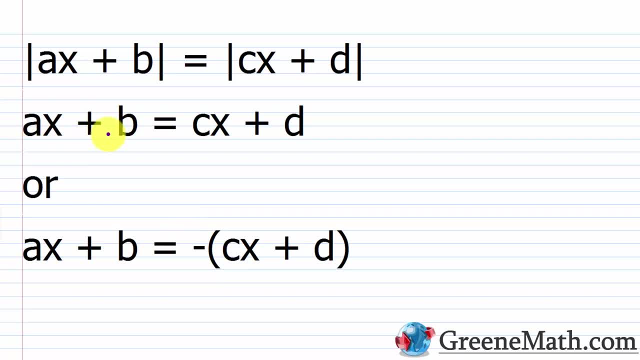 or if they're opposites of each other. So we would say ax plus b is equal to cx plus d. So in the first scenario, just remove the absolute value bars. the two expressions that were inside of the absolute value bars just equal to each other. 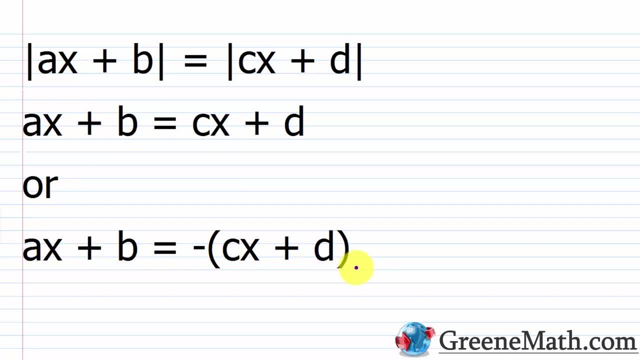 Then or next, you're going to remove the absolute value bars and you're going to put parentheses around one of the expressions and basically negate it right. So you're going to put a negative sign in front of it or make it into its opposite. You can even put this as a 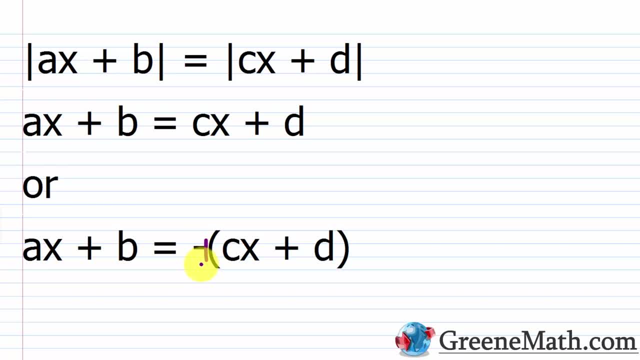 negative one out in front just to make it crystal clear what you're doing. And it would be just as valid if I said: or, and I put a negative out in front of ax plus b and said this is equal to cx plus d. Just don't make them both negative, Only make one of them negative. 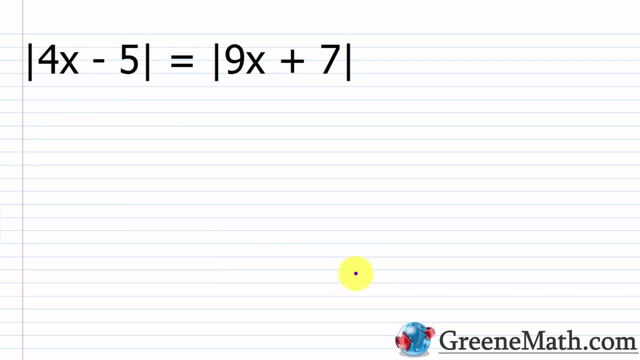 because you need them to be opposites. So let's look at our example. We have: the absolute value of 4x minus 5 is equal to the absolute value of 9x plus 7.. So again, I'm going to drop the. 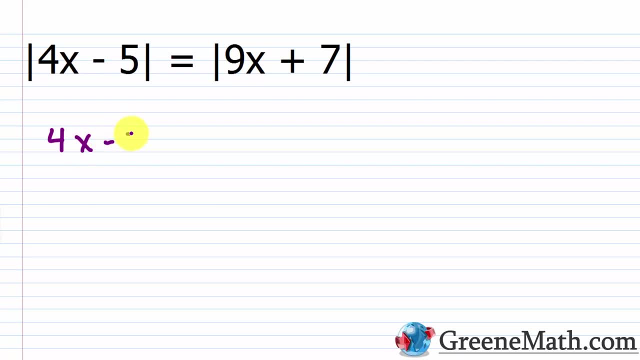 absolute value bars. So I'm just going to say this is: 4x minus 5 is equal to 9x plus 7.. So I'm going to solve that. Then you have, or you have, or I'm going to drop the absolute value bars. So I'm 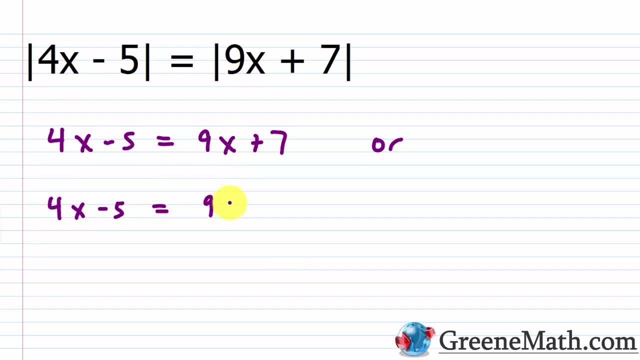 going to say: 4x minus 5 is equal to you have 9x plus 7.. So I'm going to choose one of these expressions- It doesn't matter which one you want- Wrap it in parentheses and put a negative out in. 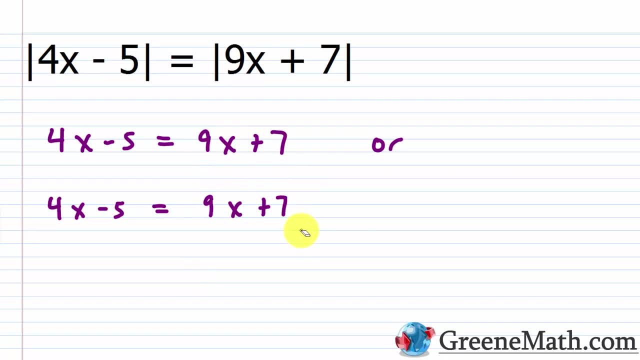 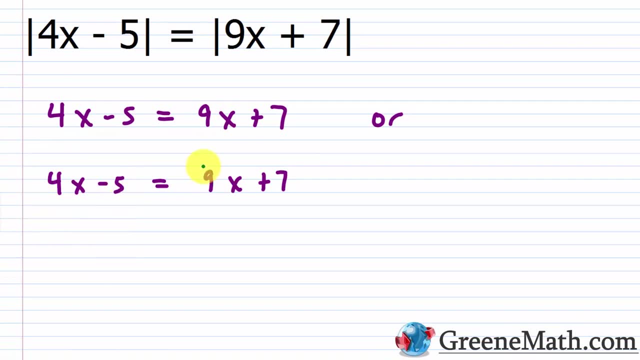 front. Okay, You could do this. one or again, doesn't matter, You can do this one, You will get the absolute same answer. Just for the sake of what we did earlier, I'm going to go ahead and just wrap this around here and just be done with it. Okay, So for the first one, I'm just going to 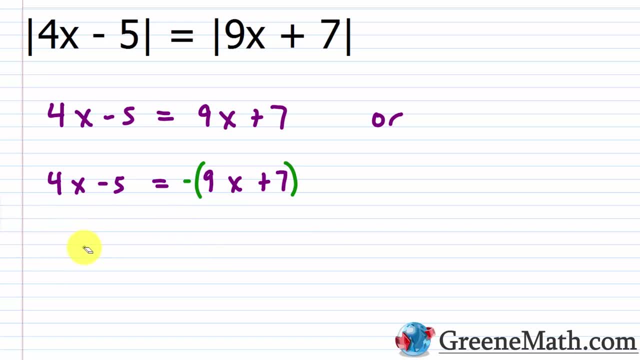 solve this. I'm going to write this down here. So we have: 4x minus 5 is equal to 9x plus 7.. So I'm going to write 4x Again: 4x minus 5 is equal to 9x plus 7.. Let me scroll down and I'll come back. 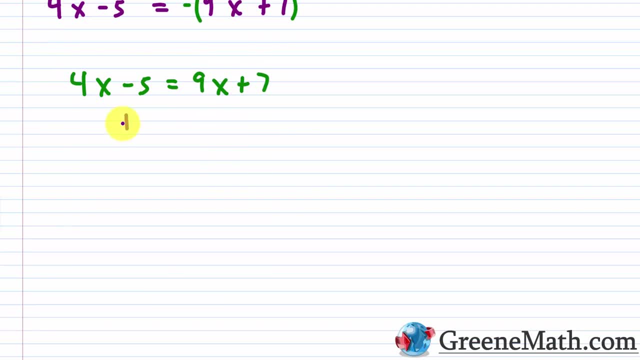 up. So to solve this is very, very easy. We just add 5 to each side of the equation. That cancels. 4x is equal to 9x plus 12.. We subtract 9x away from each side of the equation And this is going. 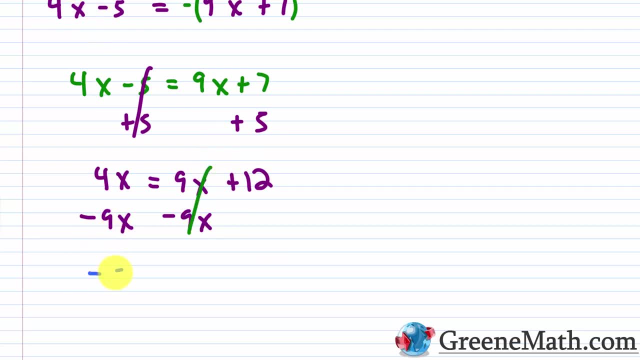 to cancel. So what I'm going to have is 4x minus 9x is negative 5x. This is equal to 12.. We can go ahead and divide each side of the equation by negative 5. And we're going to find that x is. 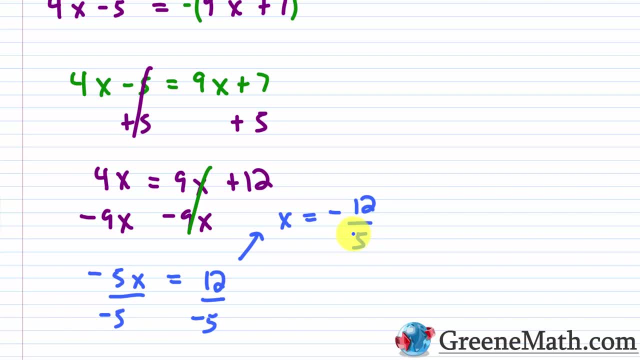 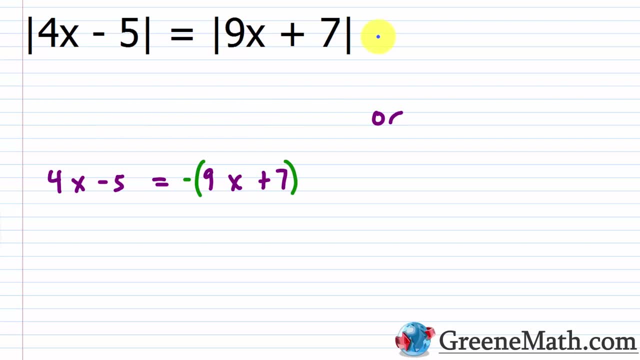 equal to negative 12 fifths. So let's erase all of this. We're going to keep that x equals negative 12 fifths, So I don't need this equation anymore. I'm just going to put x equals negative 12 fifths. 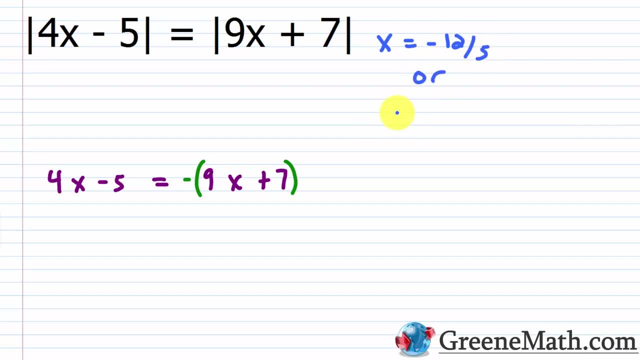 And then I'm going to have my or. here I'm going to do it vertically, And then I'll have x equals something here And we'll get that from this, Okay. So here I'm going to distribute my negative to each term. Again, if you have 12, you're going to have x equals negative 12 fifths. So I'm going